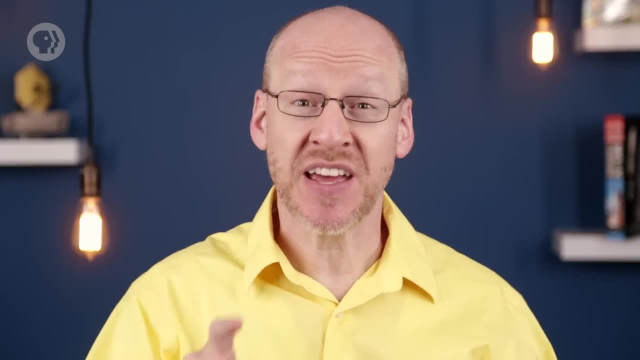 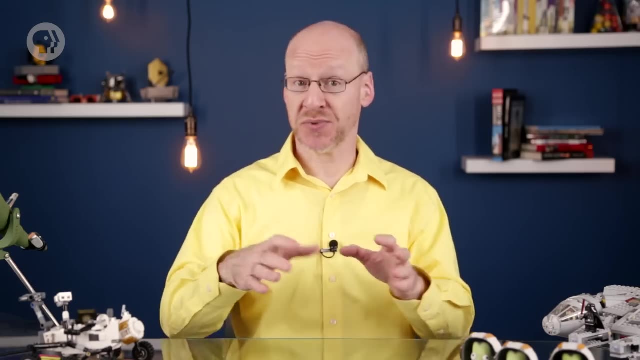 black. That might seem like the end of the story, but I skipped a step, and it's a beauty. When helium fusion stops, the Sun's core will have about half the mass of what the Sun does today. The rest will have blown away into space around it. What remains is basically: 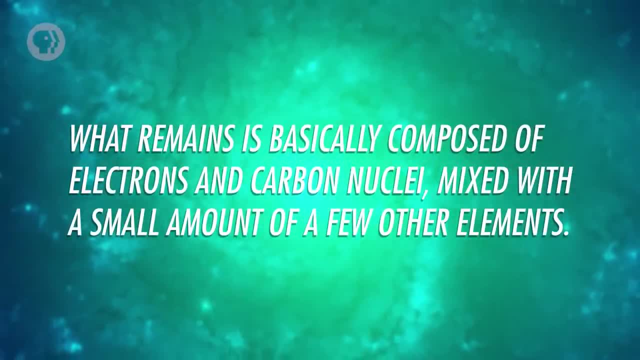 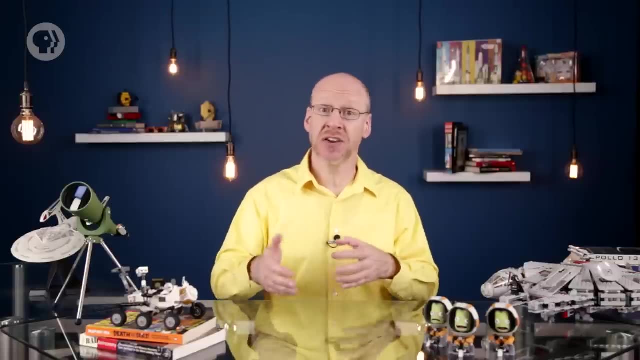 composed of electrons and carbon nuclei, mixed with a small amount of a few other elements. So what kind of an object are we left with here? You may know that light charges repel Electrons, have a negative charge and repel each other. 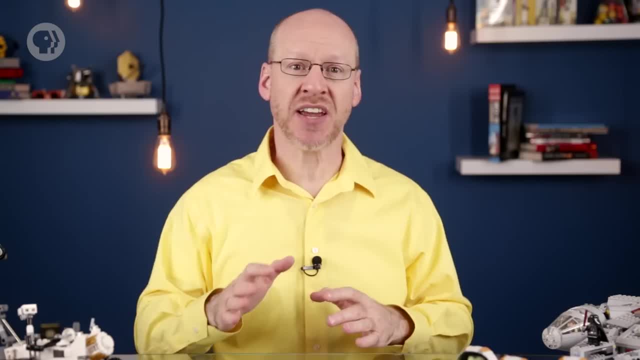 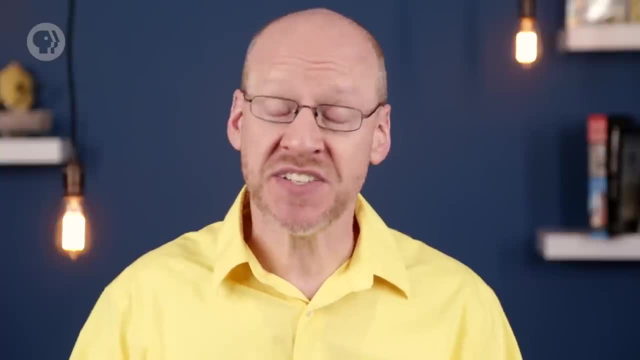 The tighter you squeeze them, the stronger that pressure. There's also a second force called a electron degeneracy pressure. It's a result of some of the weird rules of quantum mechanics. For you QM nerds, it's the Pauli exclusion principle. This describes how subatomic particles 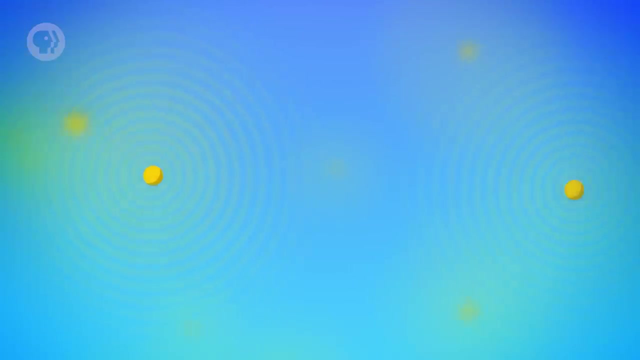 behave on teeny scales. One of these rules is that electrons really hate to be squeezed together. above and beyond simple electric repulsion, This resistance is phenomenally strong and becomes the dominant force in supporting the core of a star once helium fusion stops. By the time this electron 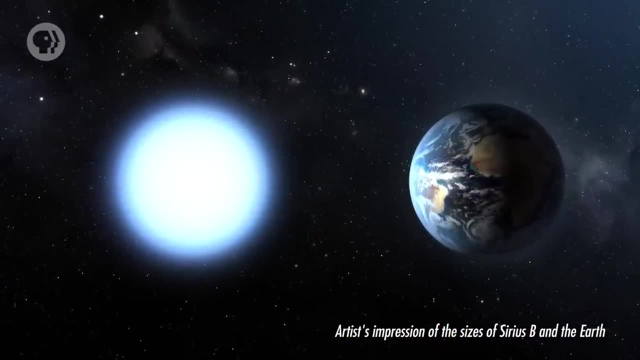 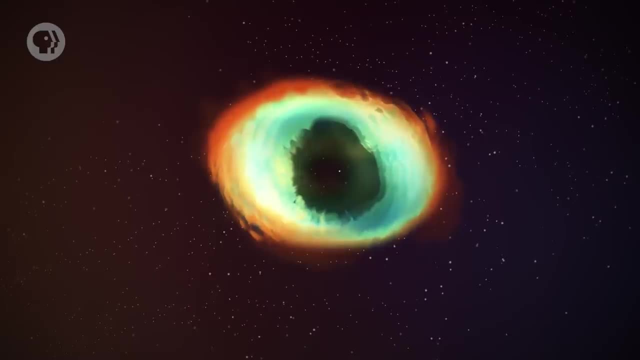 degeneracy. pressure balances the core's immense gravity. the core is only about the size of Earth- 1% the original width of the Sun- And it's called a white dwarf. Listing its characteristics is enough to melt your brain. Ironically, everything about it. 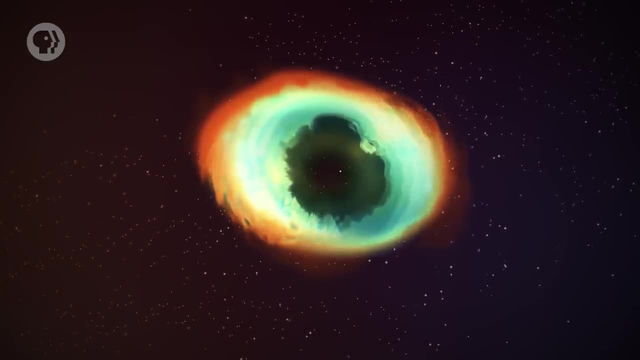 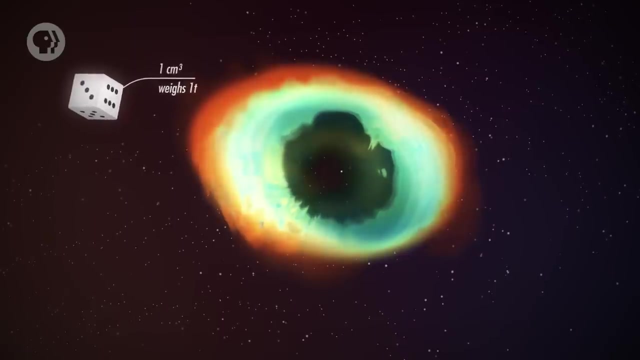 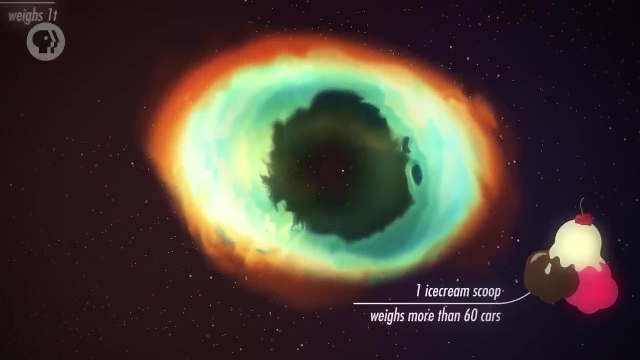 gets amplified as its size shrinks, It becomes ridiculously dense. A single cubic centimeter of it, the size of a six-sided die, has a mass of a million grams. one metric ton: An ice cream scoop of white dwarf material outweighs 60 cars, Because it's so dense. the gravity. 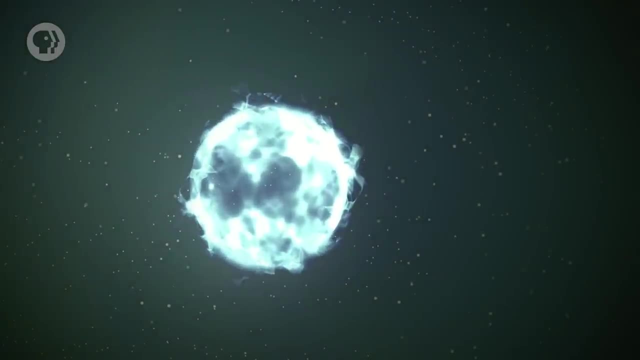 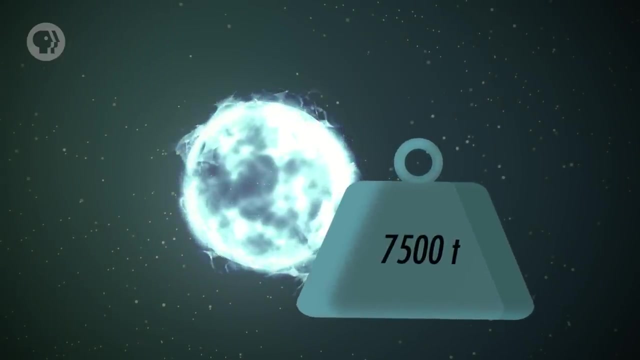 at the surface of a white dwarf screams up easily, topping 100,000 times the Earth's gravity. If you have a mass of 75 kilos, you'd weigh 7,500 tons if you stood on the surface of a white dwarf. 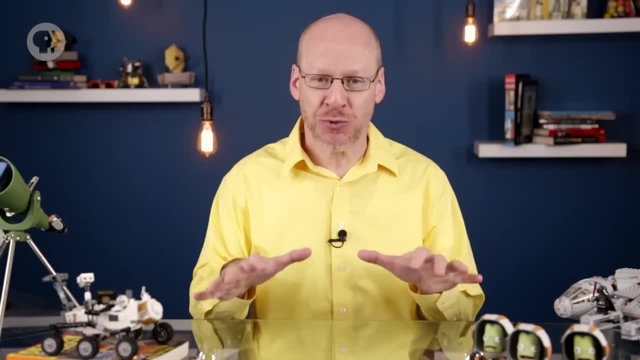 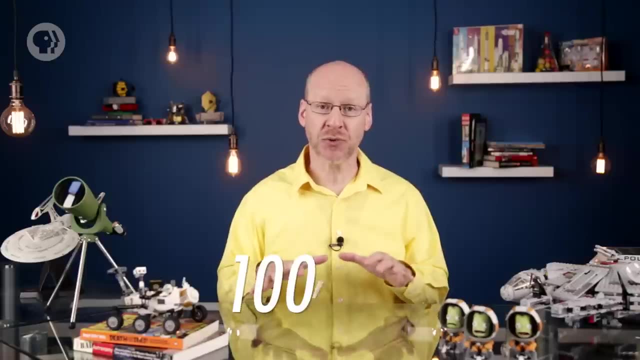 Not that you can Stand there, I mean You'd be flattened into a greasy smear, But not for long. Newborn white dwarfs are hot. They can glow at temperatures of upwards of 100,000 degrees Celsius. If you were on the surface, you'd be a vaporized and ionized smear. 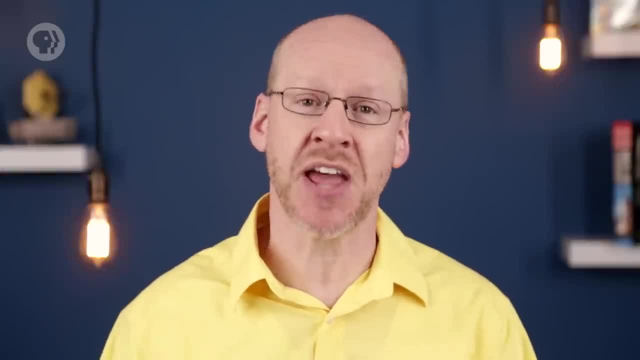 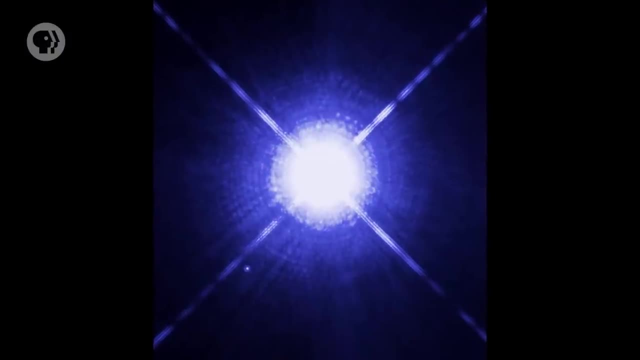 Their intense heat makes them white and they're small, Hence their name. They're so hot. they also glow in the ultraviolet, even in X-rays. Weirdly though, because they're so small, they're actually quite faint. 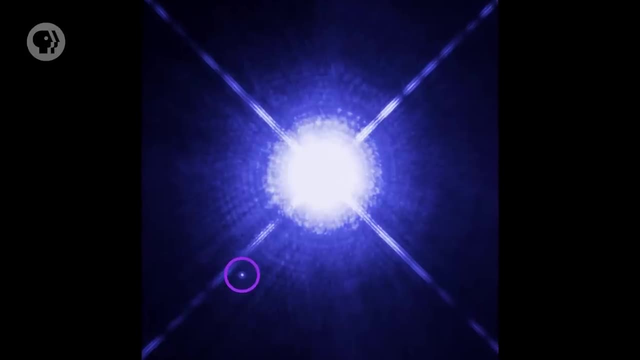 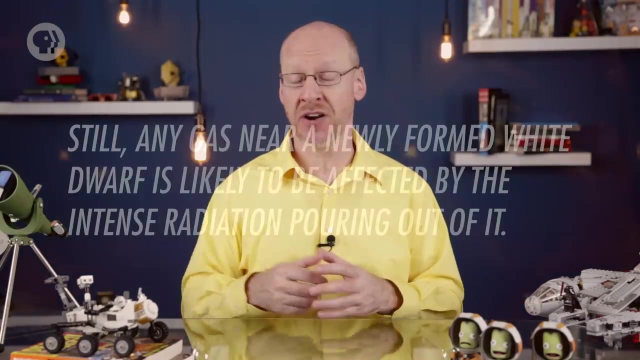 The closest one to us, Sirius B, can only be seen with a telescope, even though it's nine light-years away, one of the ten closest known stars. Over 10,000 white dwarfs have now been found in our galaxy. Still, any gas near a newly formed white dwarf is likely. 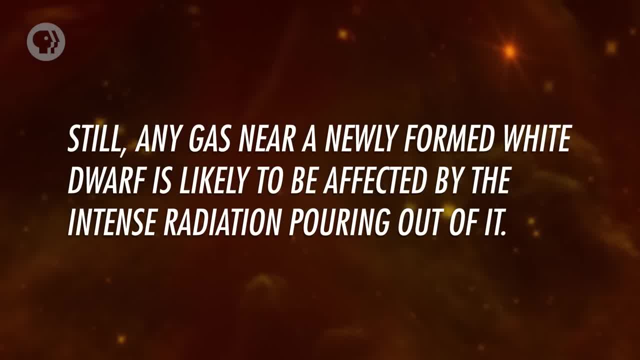 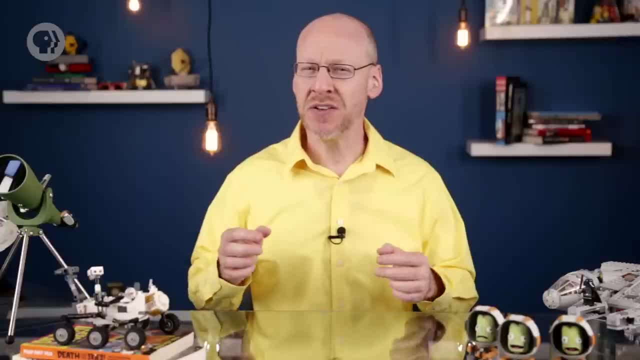 to be affected by the intense radiation pouring out of it. And hey, wait a sec. When a star like the Sun is in its final death throes, it expels its outer layers as a gaseous wind. You don't suppose? Yep, By the time that white dwarf forms, the gas blown off hasn't gotten very far from it, at most a light-year or two. That's plenty close enough to get zapped by the white dwarf radiation, causing that gas to glow. in response. 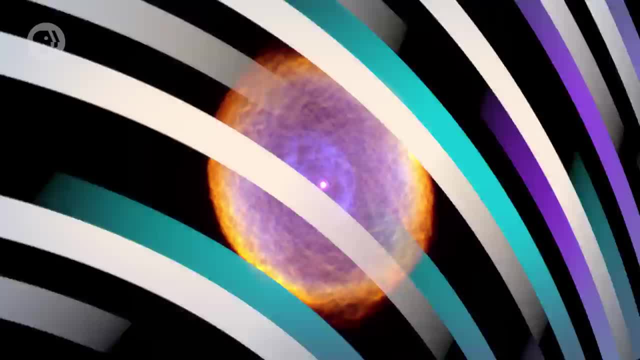 What does something like that look like? Why it looks like this? This object is what we call a planetary nebula. It's a funny name and, like so many other names, it's left over from the early 20th century, but it's still called a planetary nebula. 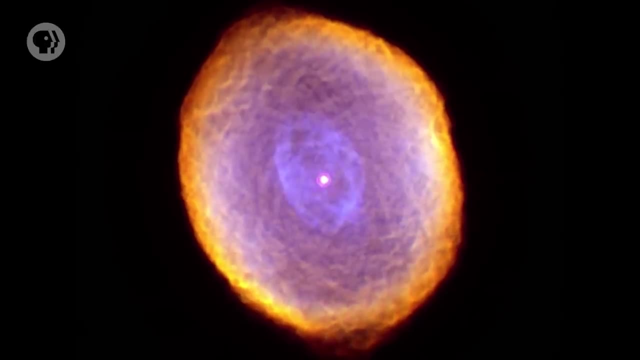 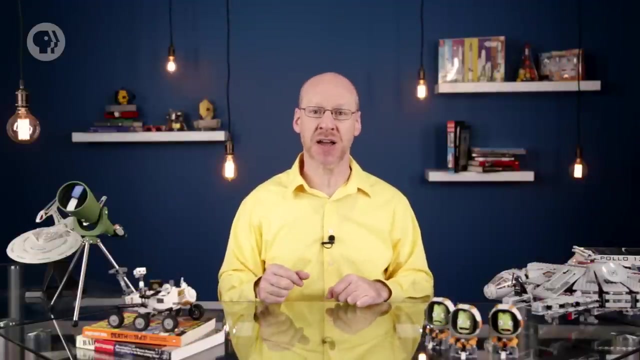 It's not far from when these objects were first discovered. The astronomer William Herschel, the same man who discovered infrared light and the planet Uranus, gave them that name because they appeared like small green disks through the eyepiece. The first planetary nebula was discovered in 1764 by the French astronomer Charles Messier. 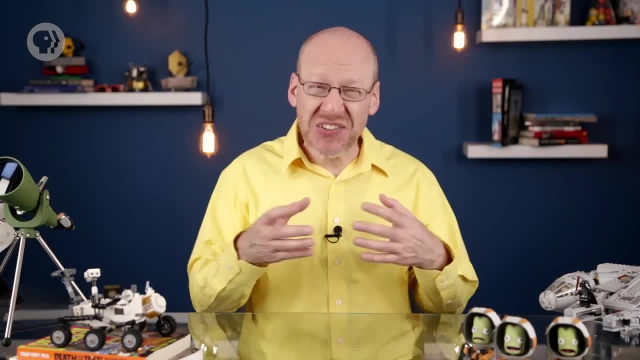 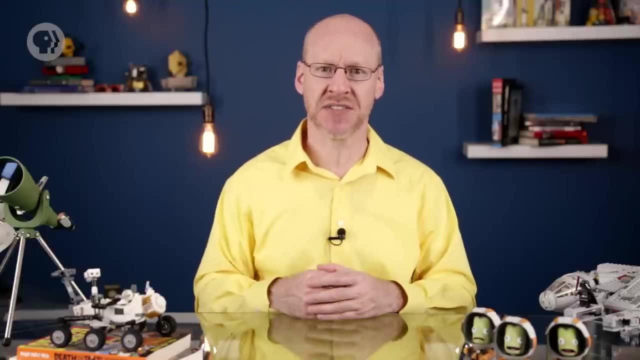 who spent years scanning the skies looking for comets. He kept seeing faint, fuzzy objects that he mistook for comets, so he decided to make a catalog of them, a sort of avoid-these-objects list. This list is now a staple of amateur astronomers because, ironically, it contains some of the best and brightest objects to observe. Among them is M27, the 27th object on Messier's list, one of the biggest planetary nebulae in the sky and one of my favorites. I love seeing it through my telescope when it's up high in the summer. 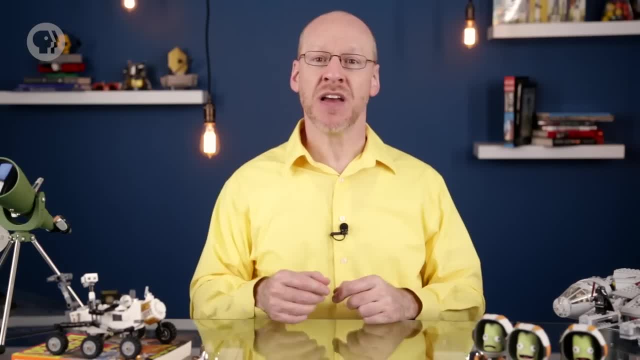 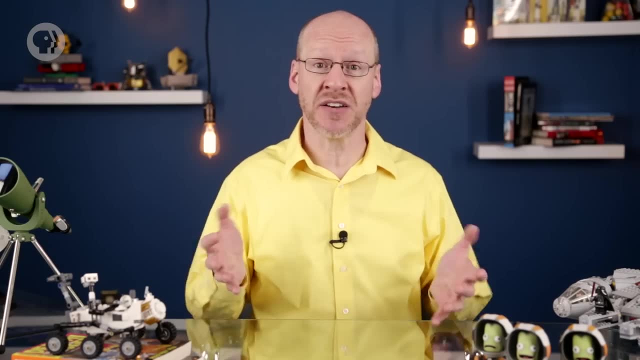 Planetary nebulae can be a bit tough to observe. Most are small and faint. On film, even with long exposures, they can appear to be little more than disks. For a long time they weren't thought to be terribly complicated. When a star becomes a red giant, it's hard to see. 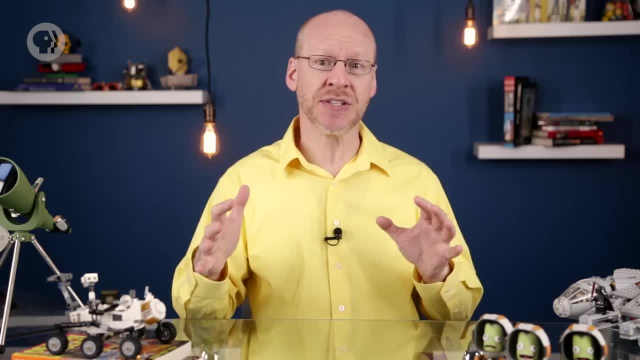 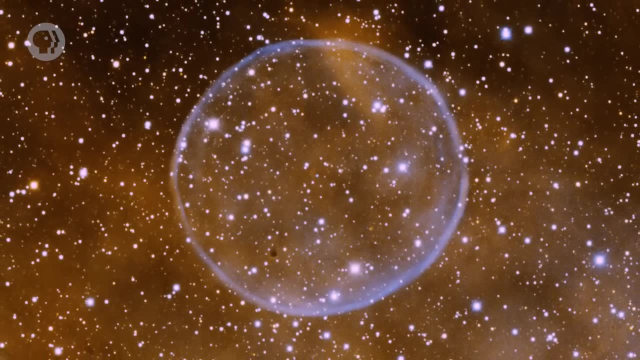 the red giant and blows off its outer layers. It's rotating very slowly, so the wind should blow away in a sphere surrounding the star. Many planetaries, as we call them for short, are round and look like soap bubbles- pretty much what you expect when you look at an expanding. 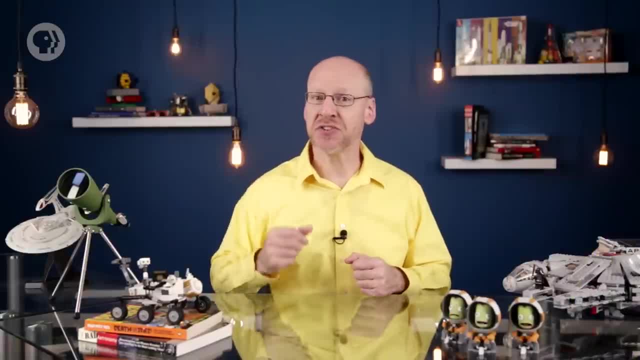 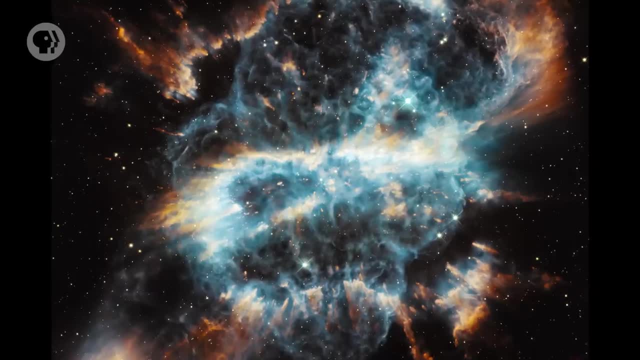 shell of gas. But with the advent of digital detectors, their fainter structures became clearer and the true beauty of these phenomenal objects was revealed. Some are elongated, Some have spiral patterns, Some have jets shooting out on either side, Some have delicate tendrils. 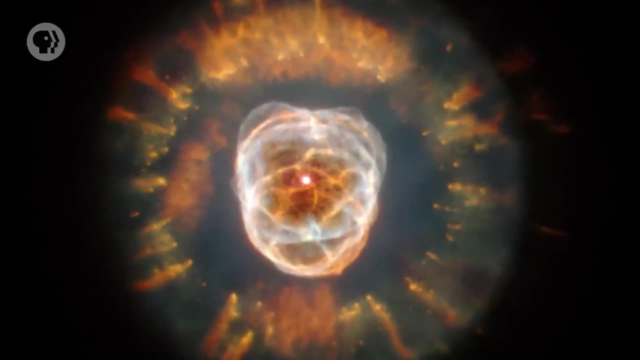 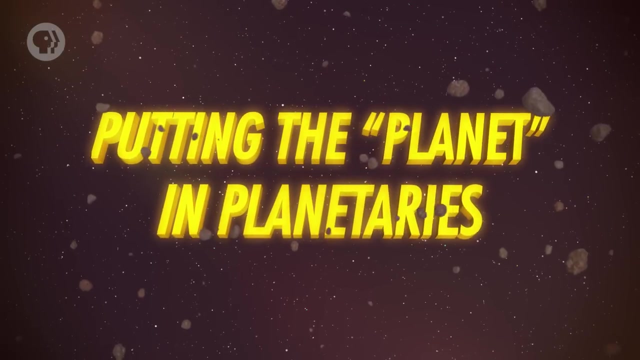 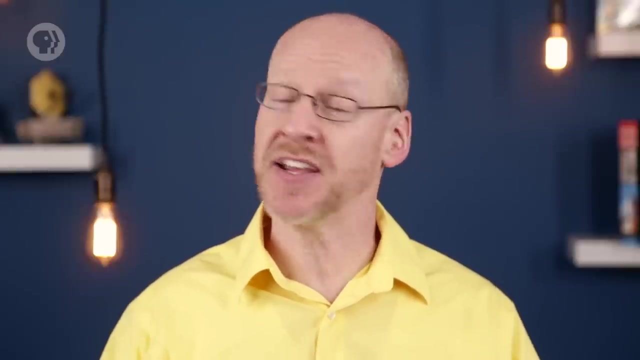 In fact, only a handful of the hundreds known are actually circular. Clearly there's more to planetaries than meets the eye. If the wind from a star blows off in a sphere, how can planetaries come in all these fantastic shapes? It turns out the real situation is more complicated, as usual When a star is. 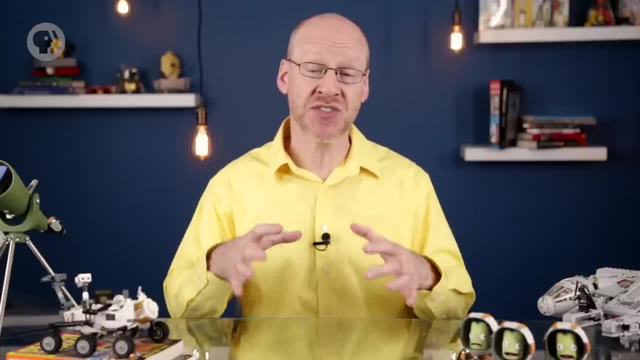 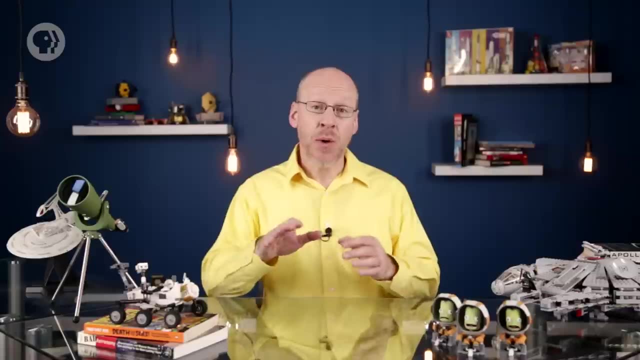 a red giant. it spins slowly and blows off a dense but slow solar wind. If there's nothing else happening to the star, then that wind will blow outward in all directions spherically. However, as those outer layers of the star peel away, they expose the deeper hotter 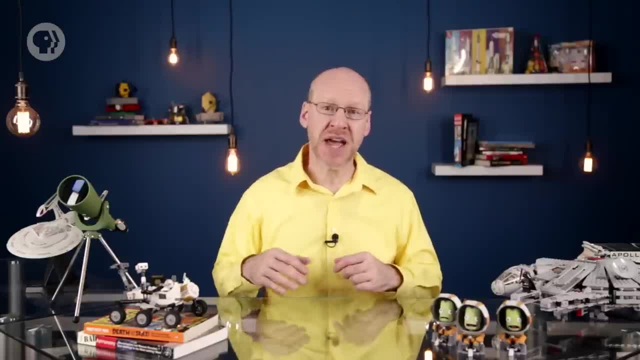 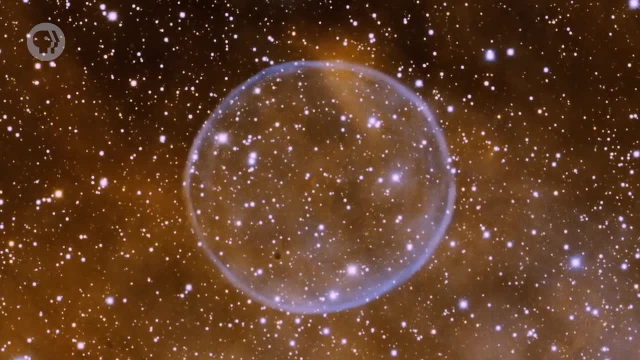 part of the star. The star starts to blow a much faster though far less dense wind. That wind catches up with and slams into the slower wind. When that happens you get that idealized soap bubble nebula. But some stars are binary. two stars that orbit very close together. We'll go into. 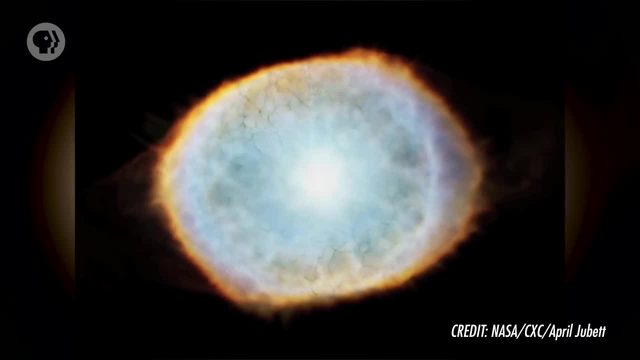 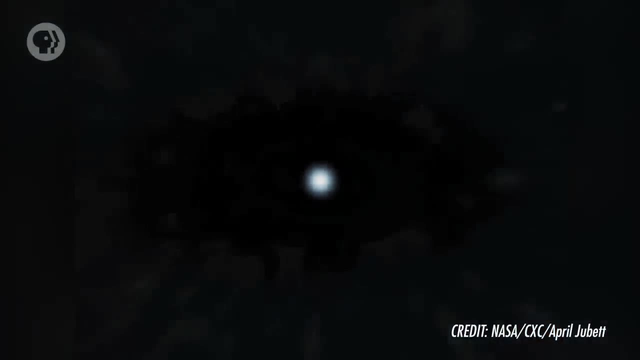 detail on them in a later episode. But if the dying star has a companion, they may circle each other rapidly. That will shape the wind, forcing more of it outward in the plane of the star's orbits. due to centrifugal force, The overall shape of the expanding gas is flattened like a beach ball. someone sat on. 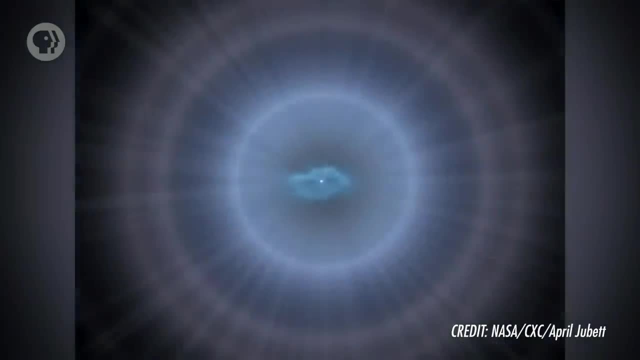 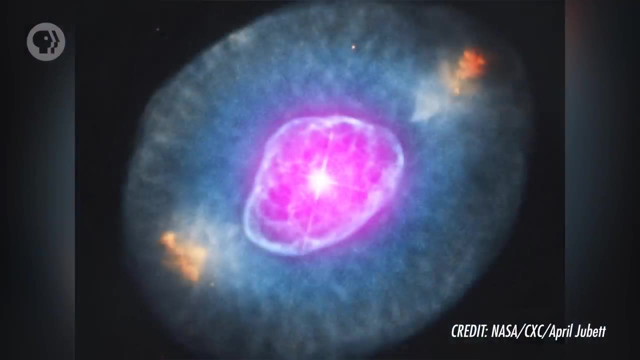 When the fast wind kicks in it slams into that stuff in the orbital plane and slows down. But there's less stuff in the polar direction up and down out of the plane. It's easier for the wind to expand in those directions and it forms huge lobes of material. 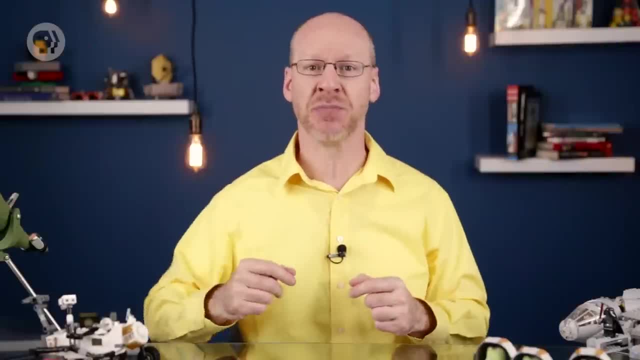 stretching for trillions of kilometers. That's a very common shape for planetary nebulae. But to explain many of the shapes we see, the two stars would have to orbit improbably close. Most binaries aren't that tight, But if the two stars are close together then they're probably closer to each other. 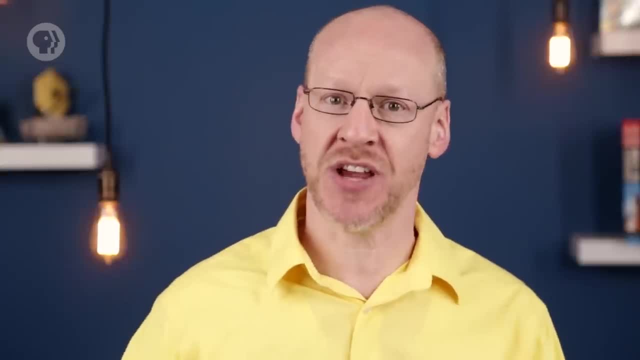 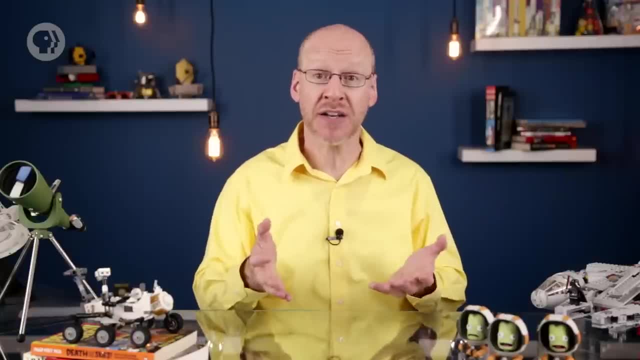 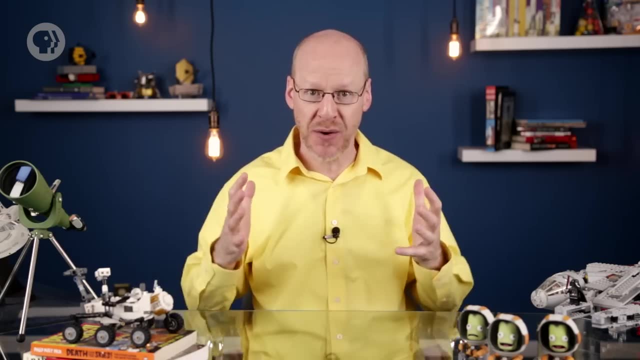 that massive planets orbiting very close to their stars were common. I suspect this is why we see so many weird and fantastic shapes in planetaries. Their progenitor stars swallowed their planets, So planetary nebulae really may owe their existence to planets. And we come full circle. The glow in a planetary nebula is due to the hot central white dwarf exciting the gas. Most of the gas is hydrogen, which glows in the red. However, a lot of the gas is oxygen. There's not nearly as much oxygen as hydrogen, But kilo for kilo. 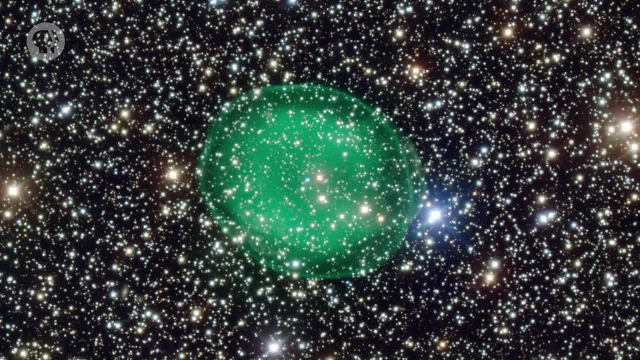 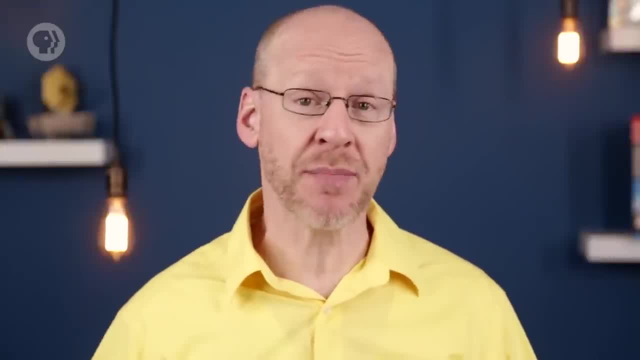 oxygen glows more brightly than hydrogen. due to the atomic physics involved, This oxygen glows green, giving planetaries their characteristic hue. Funny, When this green glow was first analyzed spectroscopically, astronomers couldn't identify the responsible element making it. They dubbed it nebulium, but eventually figured. 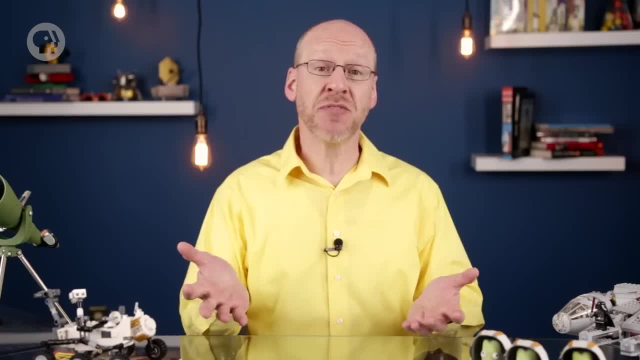 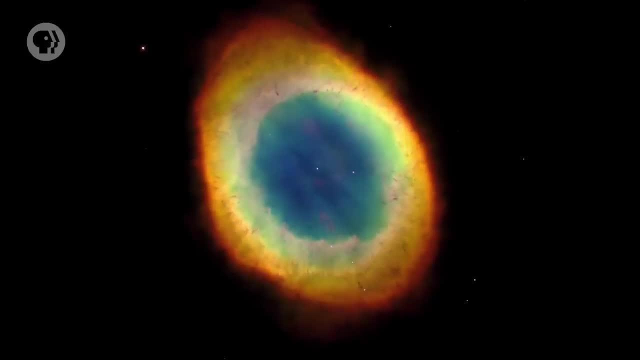 out, it was just extremely tenuous oxygen. Other colors can be found too: Nitrogen and sulfur glow red, and oxygen can emit blue as well, all adding to the beauty of these celestial baubles. But these aren't just pretty pictures: The structure, color and shape of a planetary. 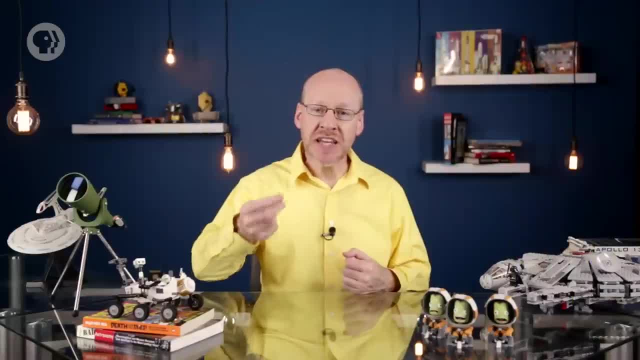 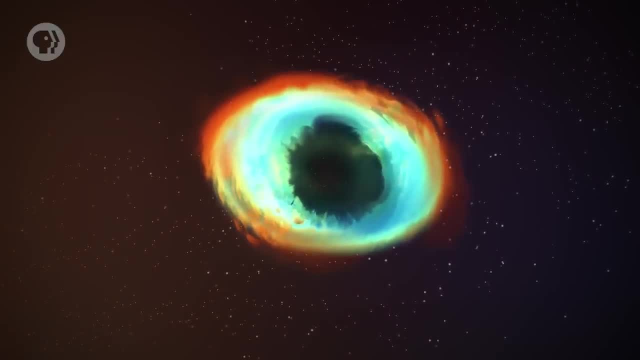 nebula tells us about the life of the star that formed it. We learn even more about stellar evolution by studying how stars die. Mind you, the gas in a planetary nebula is still expanding, cruising outward from its initial momentum of being thrown off the star. Eventually the gas expands to the other side of the nebula and the gas expands to the center of the nebula and so much it thins out and stops glowing. That takes a few thousand years. so when you see a planetary nebula, you're seeing a. 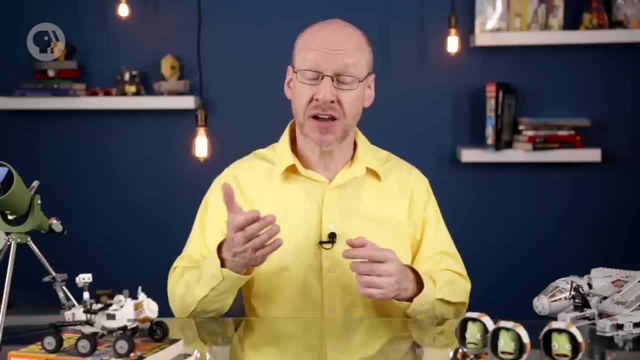 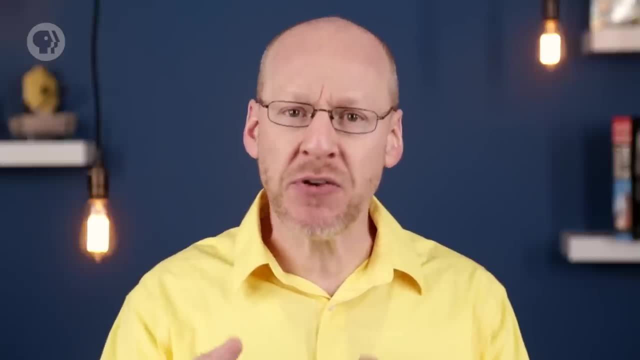 very short snapshot of the life, the death of a star, And that's why we don't see many, Though there are billions of stars in the galaxy that die this way. this phase is very brief. Enjoy looking at them while you can. And what of the Sun? Will it one day, in the distant future, be at the center of a planetary nebula? it expels as it dies. Probably not. When the Sun becomes a white dwarf, it most likely won't be energetic enough to make. 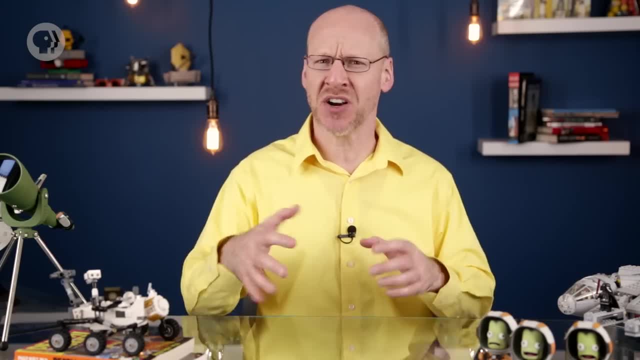 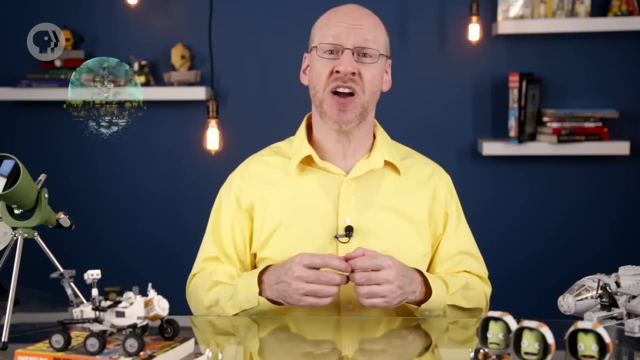 the surrounding gas glow. Most planetaries start off as stars more massive and hotter than the Sun. When our Sun dies, it'll go quietly and without a lot of visible fanfare. Alien astronomers, if they're out there in eight billion years, may not even notice. 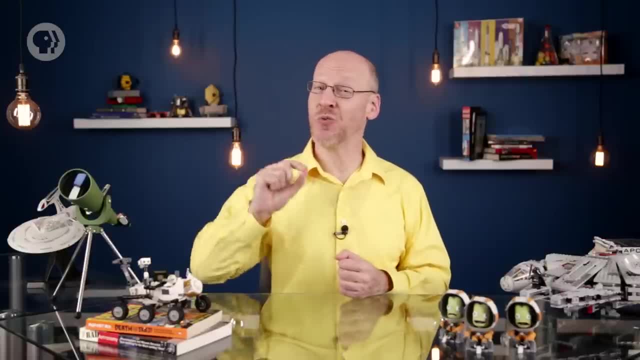 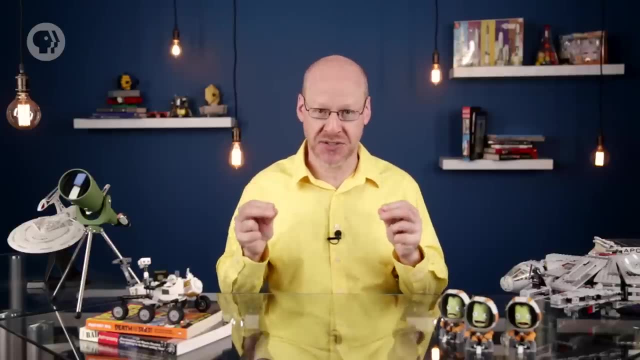 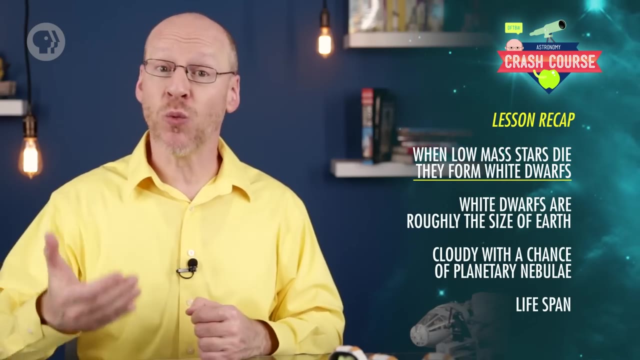 But more massive stars do make quite the spectacle, And if they're really massive, more than about eight times the Sun's mass, they really and truly make a scene. when they die, They explode, But that's for next week. Today you learned that when low-mass stars die, they form white dwarfs — incredibly. 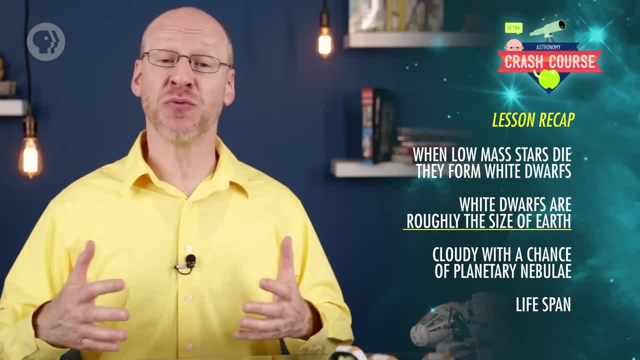 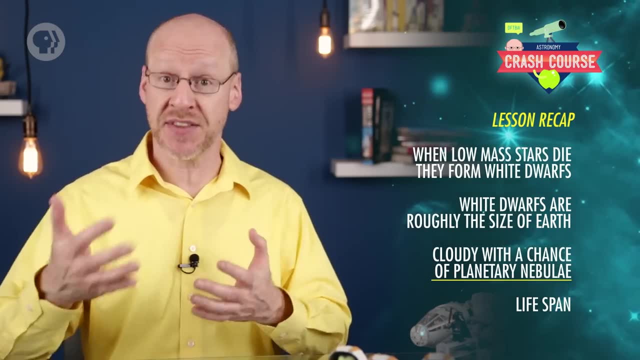 hot and dense objects roughly the size of Earth. They can also form planetary nebulae — huge, intricately detailed objects created when the wind blown from the dying stars is lit up by the central white dwarf. They only last a few millennia. The Sun probably won't. 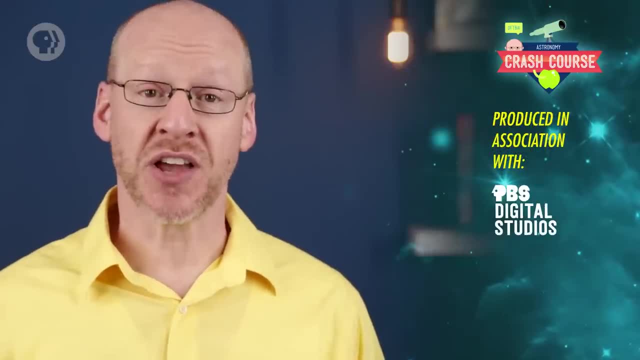 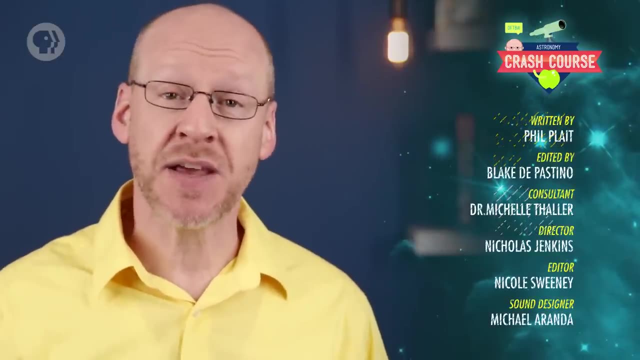 form one, but higher-mass stars do. Crash Course Astronomy is produced in association with PBS Digital Studios. Why don't you head on over there and check out their YouTube channel? They have lots of great videos there. This episode was written by me, Phil Plait, The script was edited by Blake DePastino and